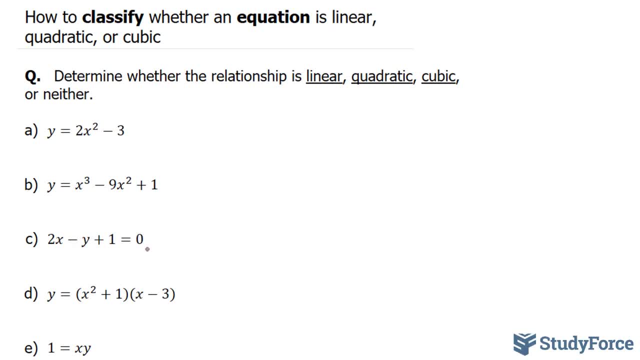 If we were to bring this y over, we would end up with an equation that looks linear. You have 2 times x. x has an exponent of 1, therefore this is linear. Moving on to D, At first glance this looks quadratic. 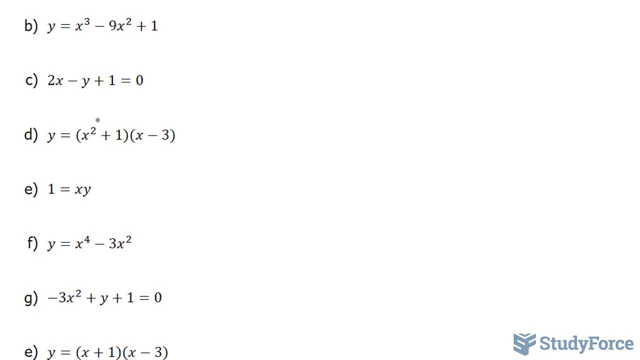 You'll notice x to the power of 2 has the highest power and you think quadratic instantly. However, if you were to expand this equation- and by expanding I mean multiplying the two binomials together- you'll notice that x to the power of 2 times x gives you x to the power of 3 as the highest power. 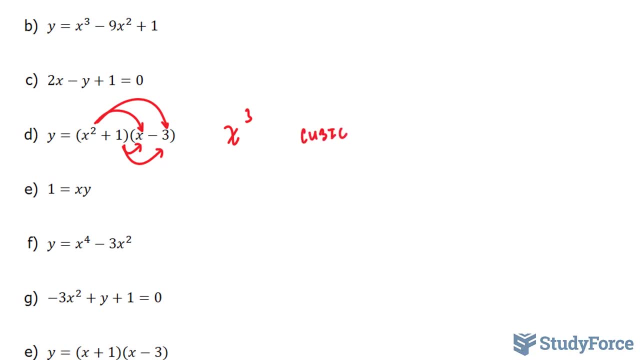 Therefore, D is cubic as well. Moving on to E, In question E we have, 1 is equal to x times y. At first glance this looks linear. However, let's go ahead and solve for y. If we solve for y, we have to divide both sides by x. 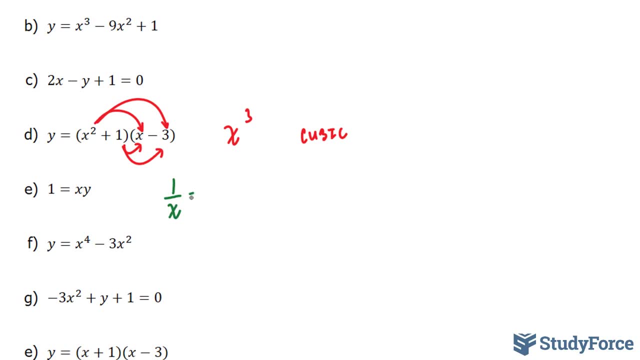 And if we do that, we end up with: 1 over x is equal to y. Now you have 1 over x and if you remember anything from the laws of exponents, this part of the equation 1 over x can be represented as: x to the power of negative 1 is equal to y, x to the power of negative 1 is not. 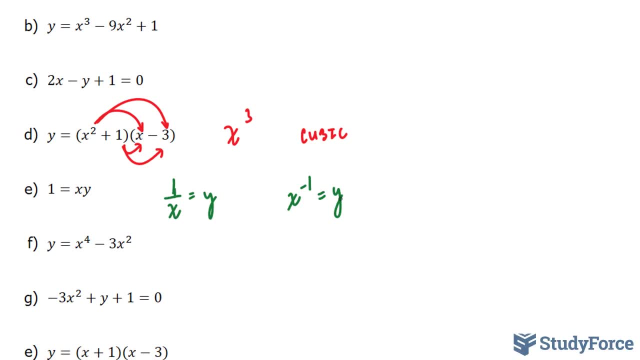 the same thing as x to the power of 1.. Obviously, negative, 1 and 1 are different, so therefore this is neither quadratic, linear or cubic. This would be something else. Moving on to f, we have: y is equal to x to the power of 4 minus 3, x to the. 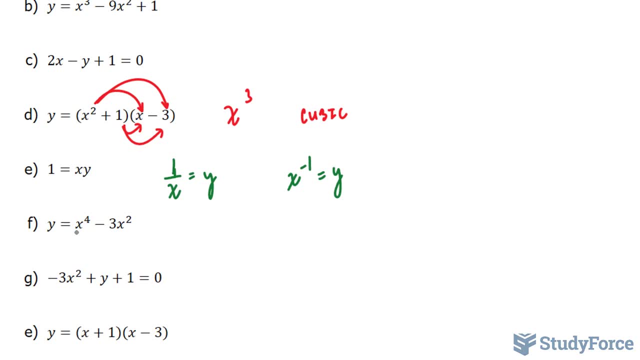 power of 2.. Here we have x to the power of 4.. x to the power 4 is neither linear, quadratic or cubic, so this would be neither as well. Moving on to g, In g we have negative 3. X squared plus y plus 1 is equal to 0.. If we rearrange this and 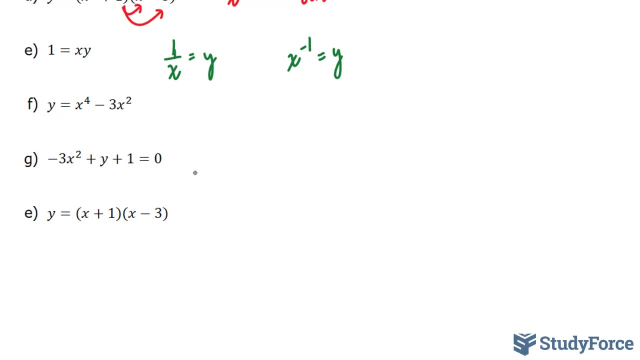 bring the y over, we end up with a quadratic equation. We have x to the power of 2, has the highest power, and so therefore this is quadratic. And lastly, at first glance this equation appears to be linear. Notice that you have x with a power of 1, and usually, 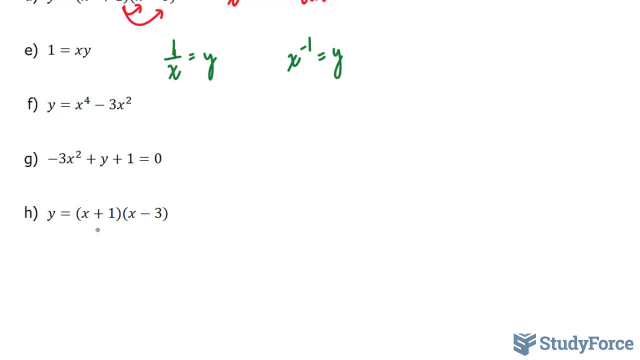 when you have a power of 1, you don't show the power, and so you're tempted to think it's linear. But if you were to expand this equation where you have x times x, x times negative 3, and so on?